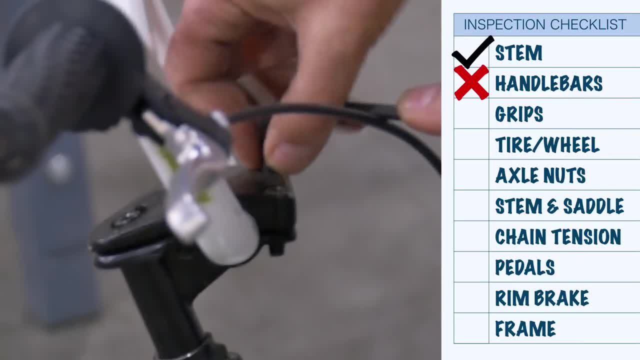 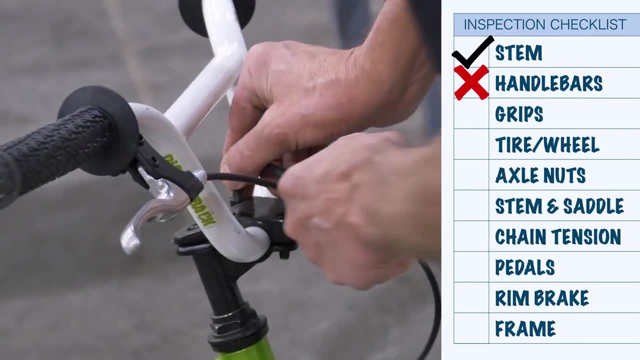 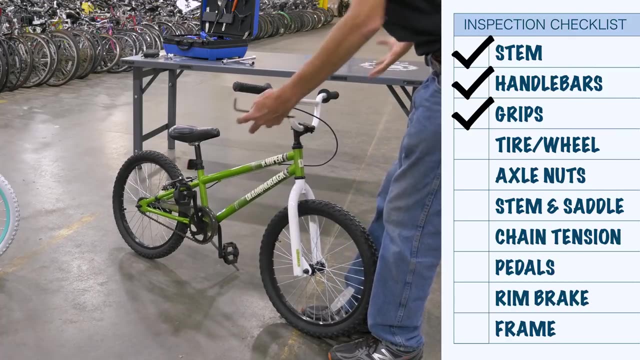 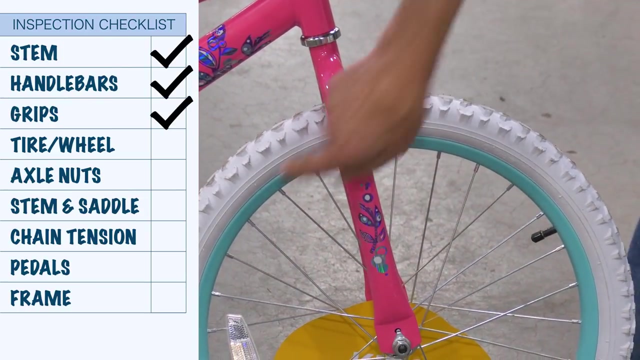 that's good. We come to the front. we tighten in a cross pattern, always going over the bars. that's good. Grips seem good. front end done. We're going to see if the tires seem reasonable. squeeze, they do seem inflated. We check around the bead: they do seem properly. 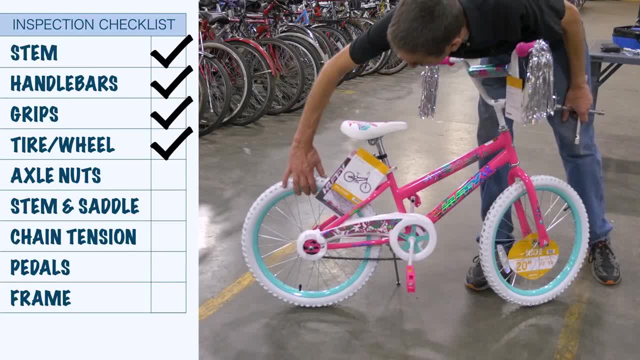 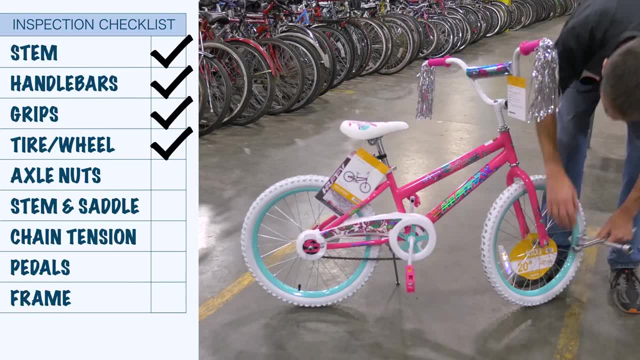 seated. We want to see the rear. it's also fully inflated. Are these wheels tight to the frame? We get a wrench out. Yes, that's tight. Yes, that's tight, Tight, tight. With a wrench like this, we're pulling on both sides, so we'll 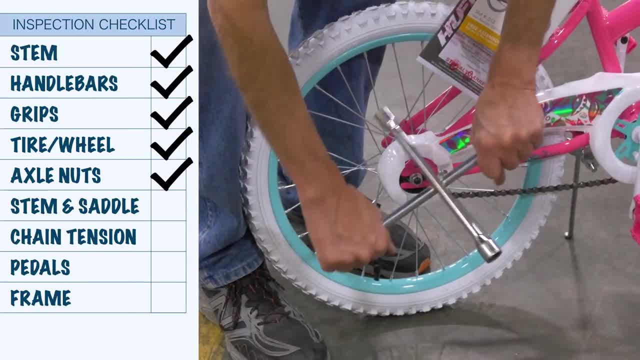 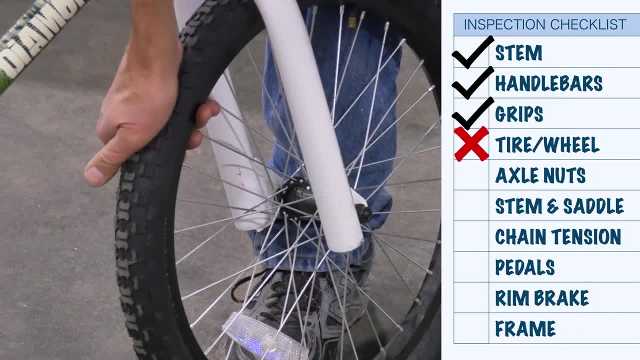 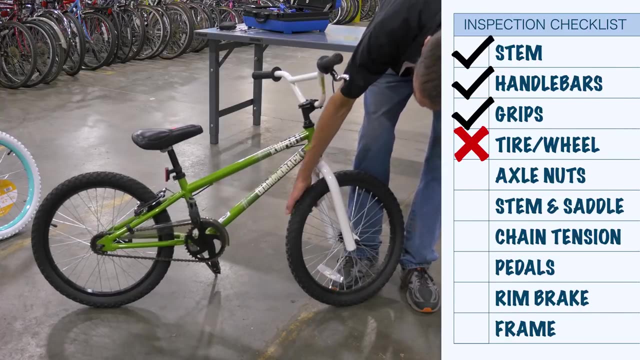 only need about 20 pounds of effort at the end of the wrench to get that tight On here. the tire does seem low so that might be a slow leak. It just might need air. The tire does look good. There's no cracking. The tread looks good, but definitely low on air. The rear one seems fine. 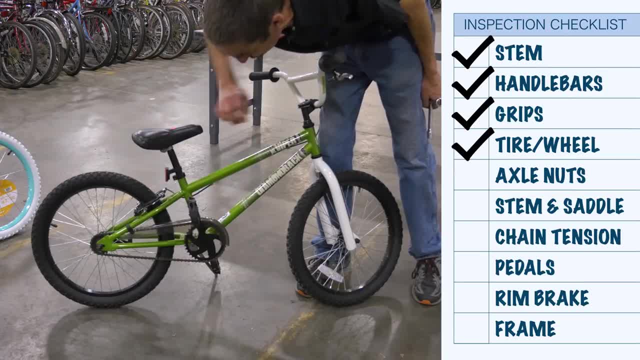 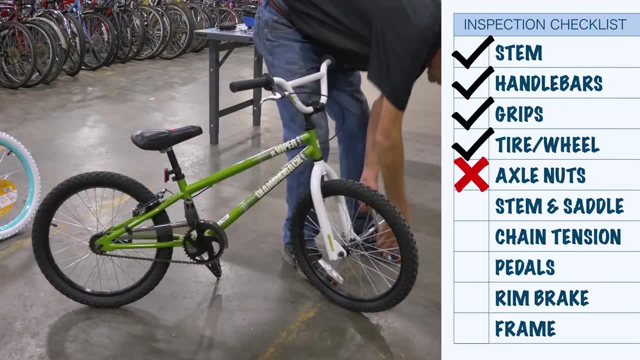 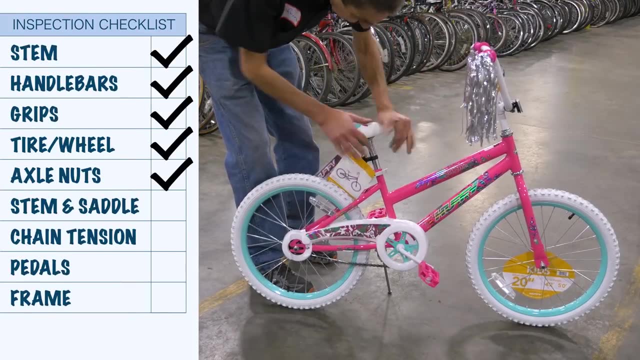 Good pressure, bead-seated, good tread Wheels. put a wrench on it? Oh, definitely loose. So we go and check all other nuts At the back end. we're going to grab the saddle, Pull up and down. It doesn't move. Left to right, it doesn't move. Saddle must be tight. 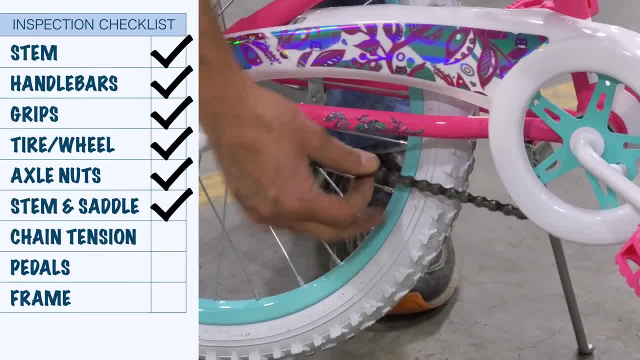 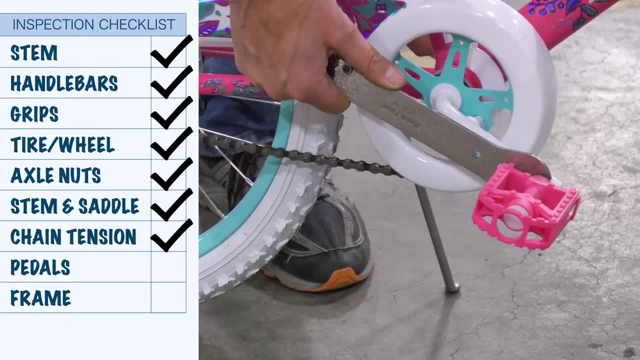 Down to the chain. a slight bit of play. There's no way that's coming off. so that's a safe chain. Are the pedals on tight? We put a wrench on, We pull up here again about a 20-pound effort on this. 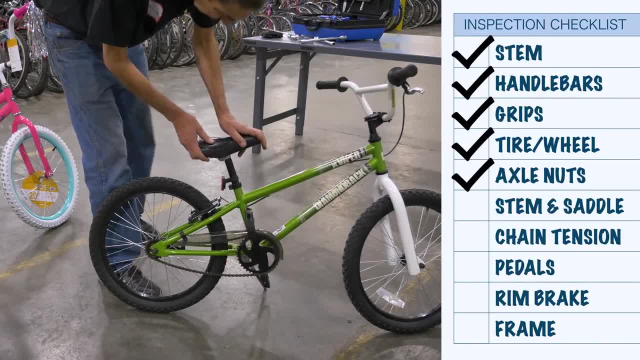 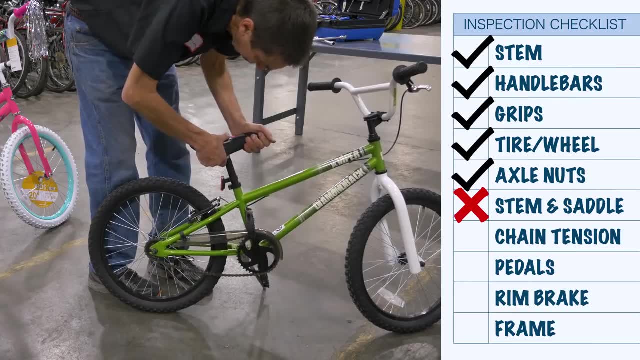 long wrench will do the job On this bike saddle. grab it. We pull up and down. Seems okay, Left to right, that's loose. Straighten it up. This isn't moving, This was moving. We come up here with the. 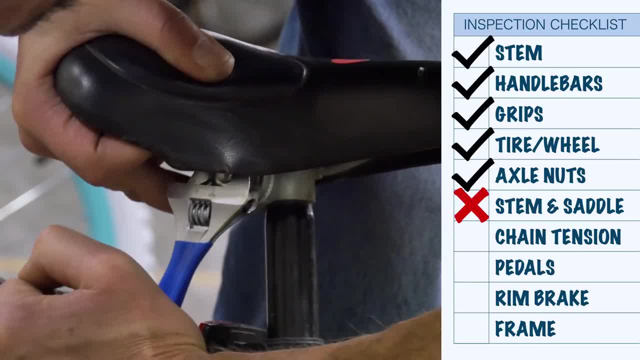 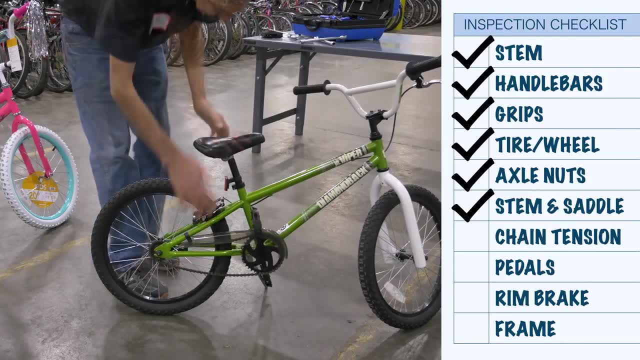 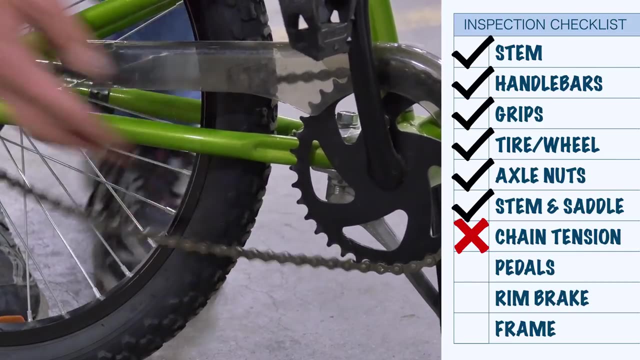 wrench. Now it's not moving. This isn't moving. This isn't moving. That's done. Next we check the chain. In this case really loose, So loose. it could come disengaged from the ring If the coaster brake was.